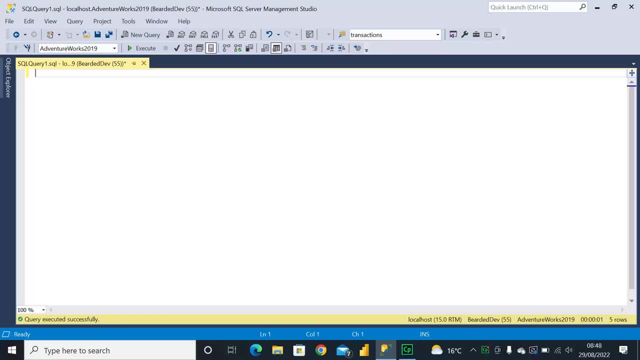 Hello and welcome to my channel. I am Bearded Dev and in this video we're going to be taking a look at how we can search the text within a stored procedure. Now, because the database isn't really self-documenting, it can be difficult when there are hundreds of tables and hundreds of stored. 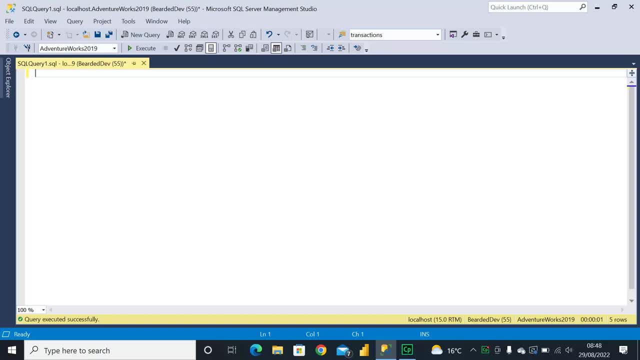 procedures or different objects involved to understand what's actually performing operations on those tables. or simply, we may want to search stored procedures just to identify which stored procedures are performing inserts, updates, deletes. Now we're going to be taking a look at the employees data within AdventureWorks 2019 within this video and one approach: say, if we 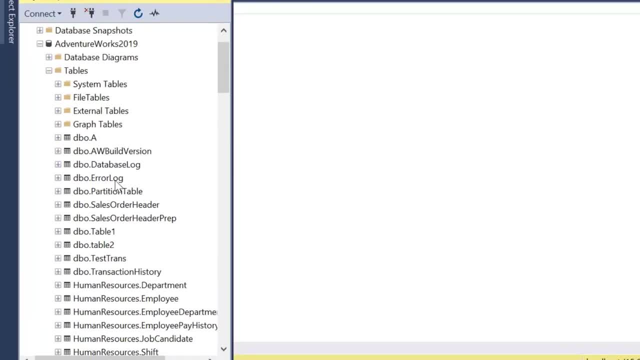 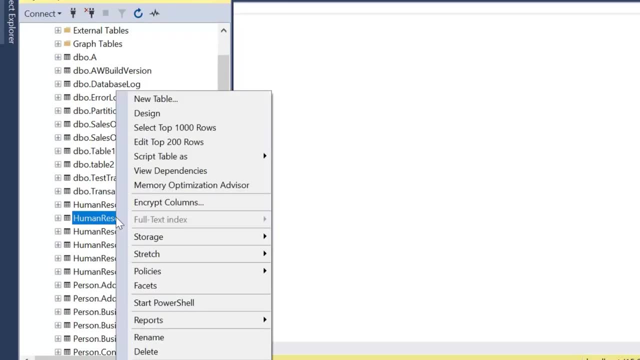 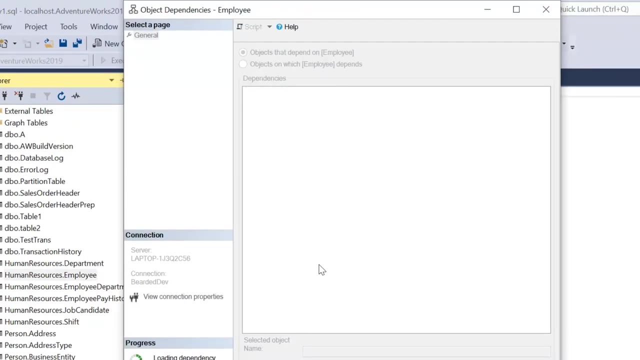 wanted to look at a table. I've opened up Object Explorer here, So if I wanted to have a look at the human resources employee table, I can simply right click on that and have a look at view dependencies. Now, if I click this now, it's going to start loading up objects that depend on employee table and we can see. 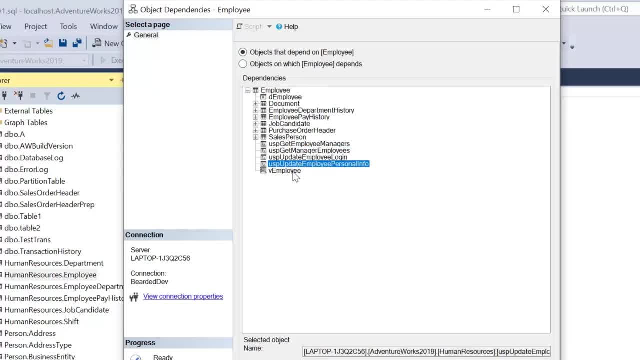 here there's a couple of different stored procedures in the list, as well as views and other tables or objects, and then we can switch that round on objects on which employee depends. Now there's a. there's a couple of problems with with this approach. The first: really I'm not convinced. 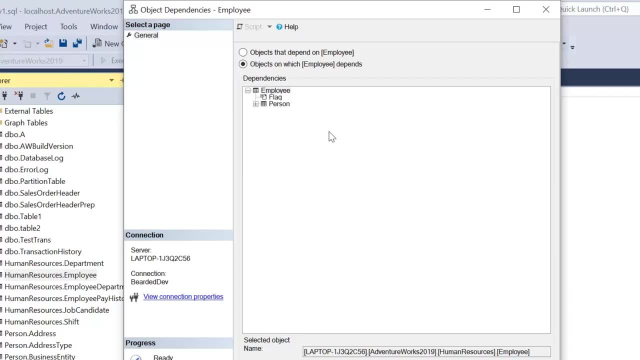 this is accurate. having worked with this over time for a number of years, I have seen objects that are missing from this list, so I never take this as gospel. The other is it does include all objects. there's no way to apply any filters to this list, it's just simply. 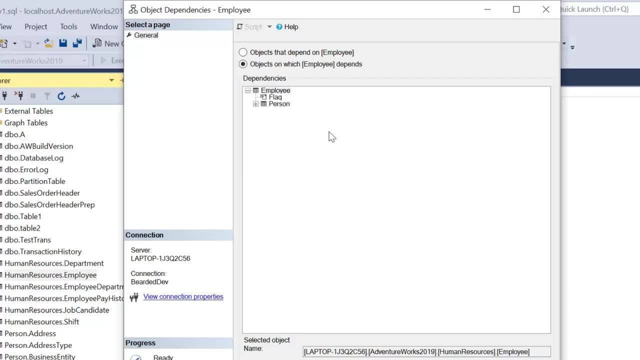 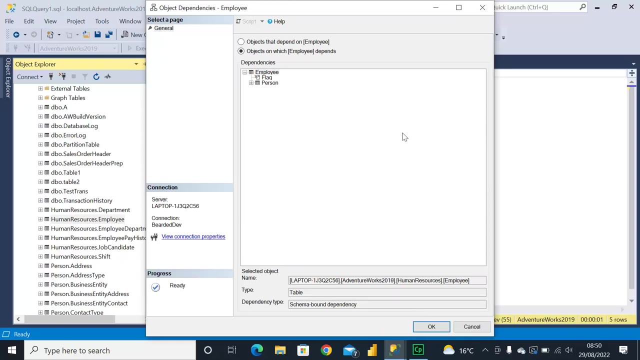 a list of objects. So what's a what's a better solution? How can we look at any stored procedure that perhaps references this table in any way? Now, within SQL Server, Azure SQL Database and Synapse Analytics, there is a catalog view, a system catalog view called syssql. 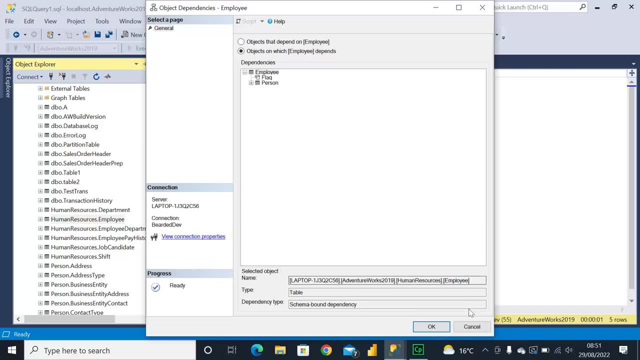 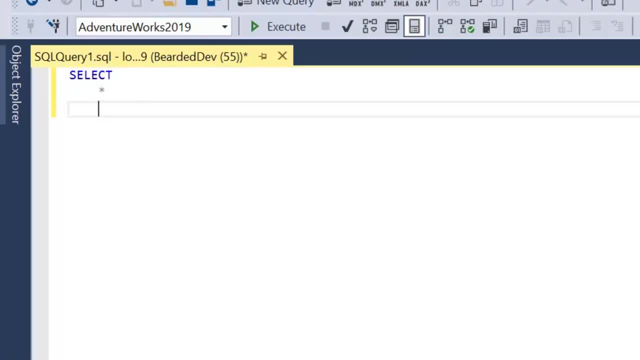 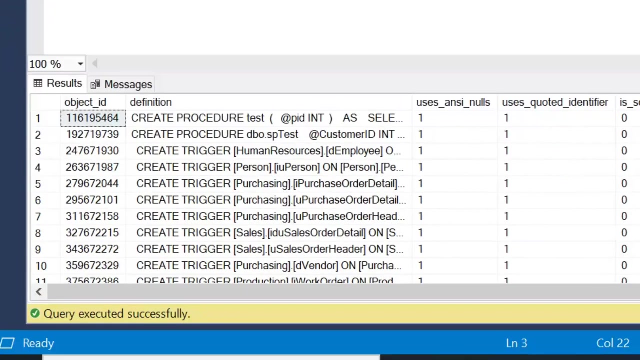 underscore modules. So let's take a look at that. Let's just do: I select all from that view to start with, select all from syssql underscore modules. Let's run that query, have a look at the what the results look like. Now this will return a row for each module defined. and what do I mean by module? 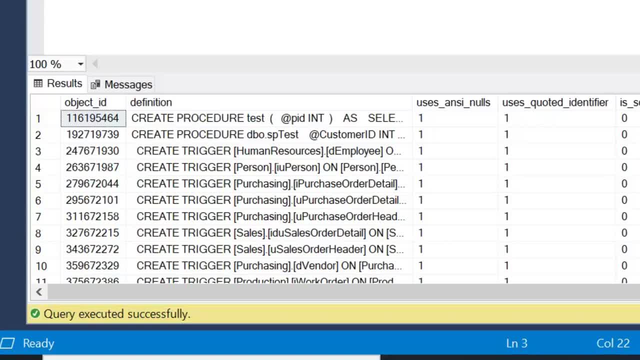 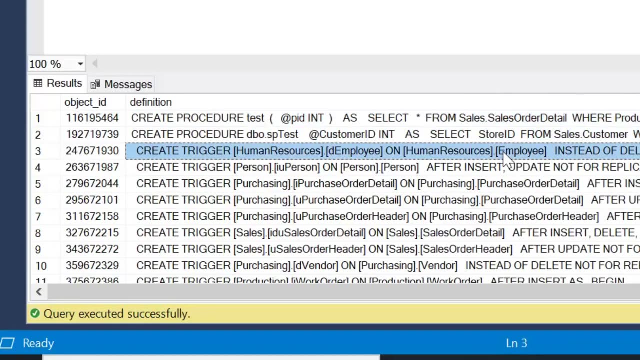 So module could be stored, procedure, trigger, view, function, anything we've defined within the database, And we can basically run all through vams. And if we take a look at this definition column here, So this is the textual representation of that object, wich is great for us because it means we can actually search the 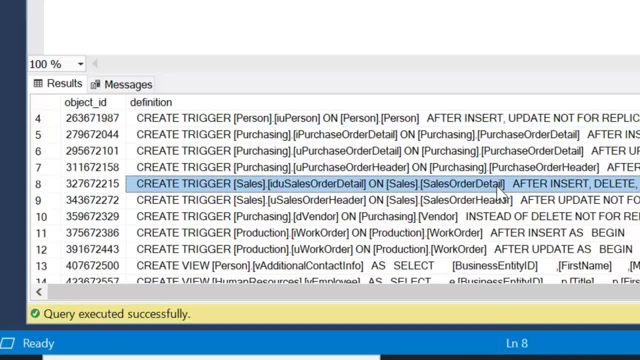 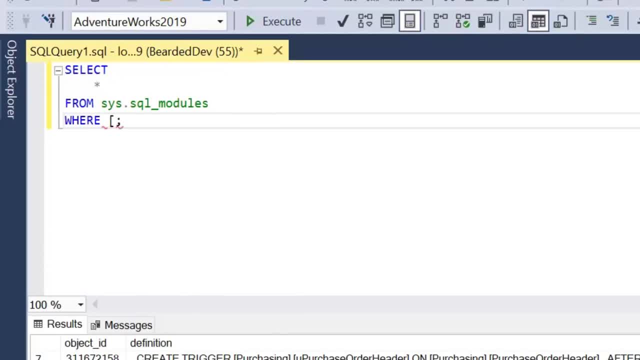 text of objects to identify anything that's referencing this table or performing seartan operations. So how I can search this is simply just having a look at. way is like employee and we are searching quite large text strings here, so it's not going to. 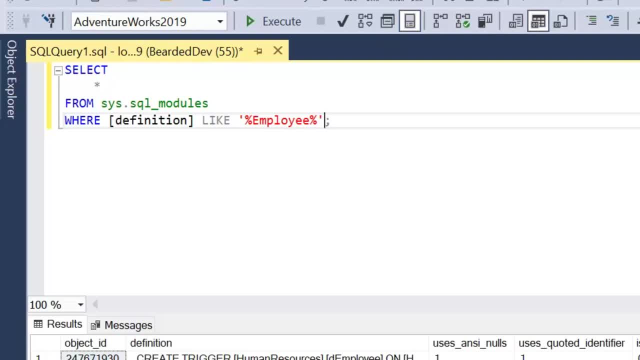 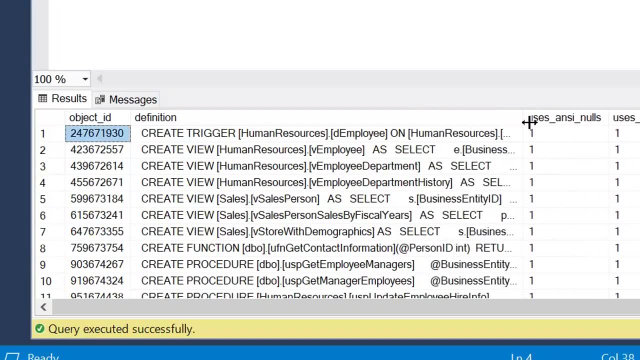 be amazing in terms of performance, especially if you've got a massive amount of objects in your database. so if i have a look at that, i can see all of these objects that reference employee in some way. so we can see: here we've got a trigger, we've got some views, we've got a 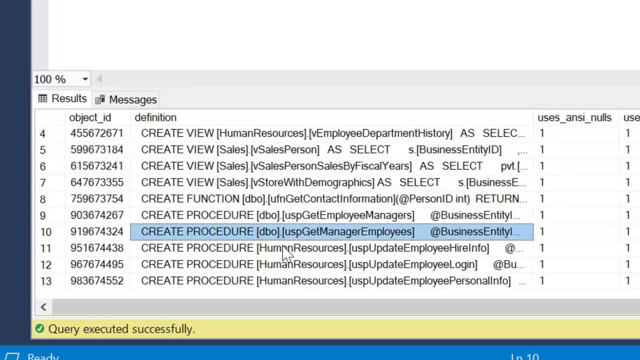 function here and we've got some stored procedures as well. now how could i filter that to have a look at different types of objects? now we can. we can tell from the definitions that's a trigger. these are views. the bottom are stored procedures. but what we actually want to do is something that 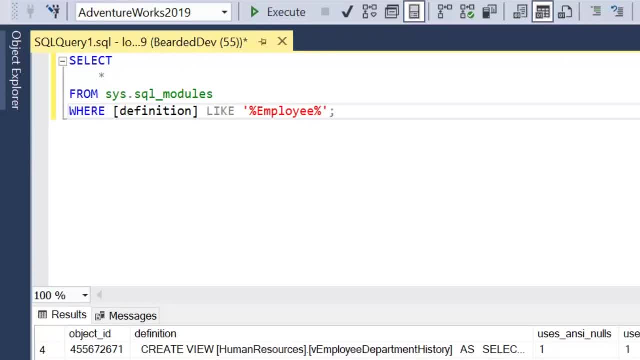 identifies them in some way. so we're going to introduce another catalog system view, which is sister objects, which will store all of the objects in the database. i'm going to join that to sql modules on object id so each object within the database has an object id, similar to how we'd 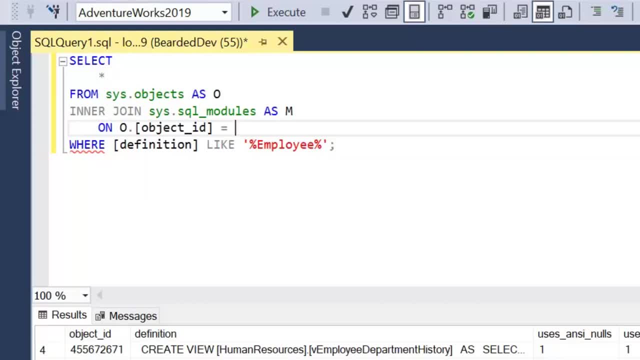 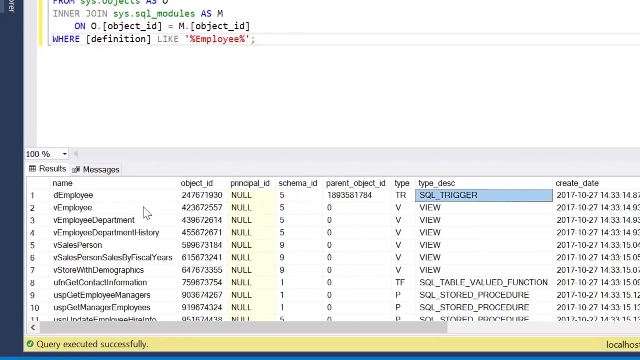 identify everything with keys. object id is a unique identifier and i'm just putting object id within a square brackets as it's a recognized keyword. so if i go ahead and perform that joint, we'll notice here we've now got the name of the object, so that's a bit better to what we 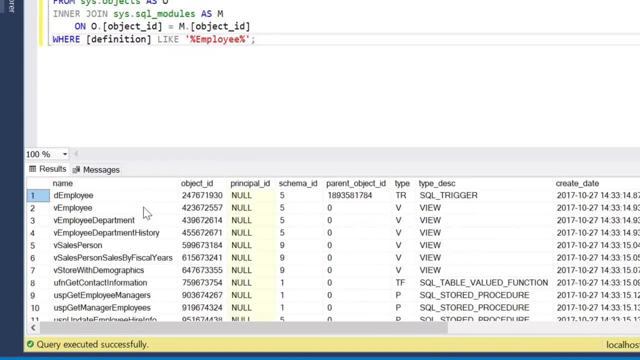 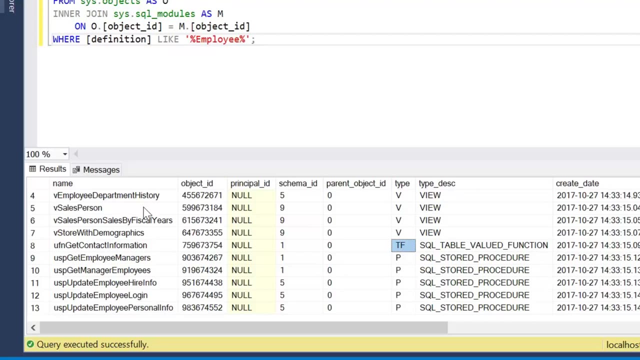 had before, rather than just the object id, but we also have this type column so we can see triggers are represented by tr, views by v. functions have a few different, so table valued functions, tf, inline functions, if so on, and then stored procedures simply as a p. so if i just 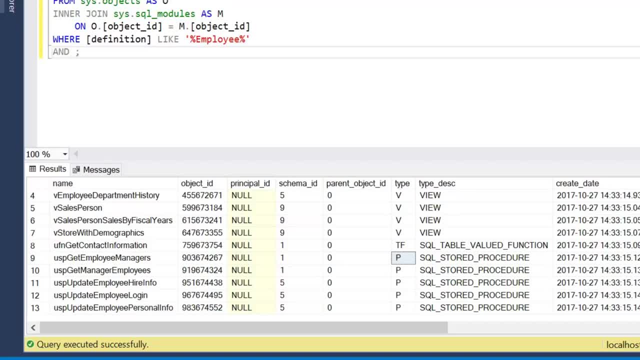 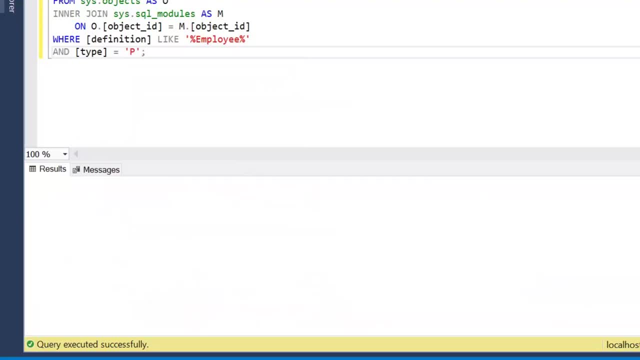 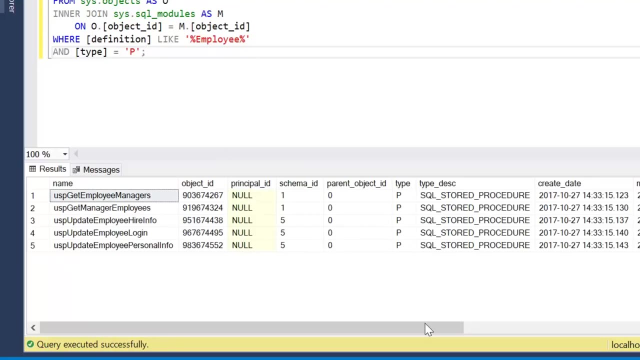 wanted to look at stored procedures. i can simply filter on that type column and again, type is a keyword, so type equals p. execute that and again we've now got it filtered to store procedures and, don't worry, if you don't like that word, we can disappear. the following way: 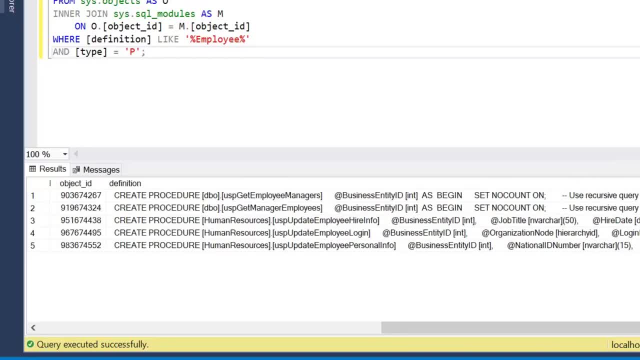 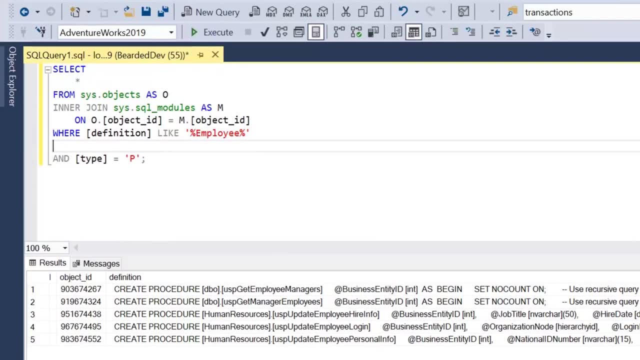 so one of the other clever things that we could do is we could be able to change the definition of the text to something like insert. so in here we can. we can change that to another display component, and now we can add the query that we were looking for, and we could be specific about this. so you have to be 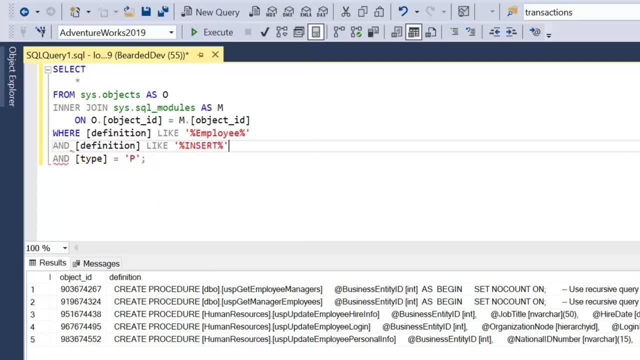 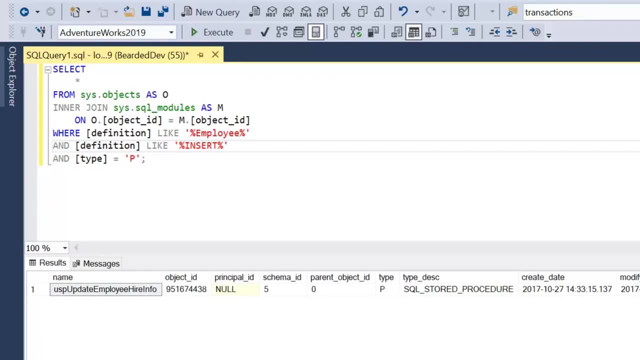 quite clever. remember. this is searching text so we could add in another search on our definition what I mean about being clever. so this: the criteria have got here. we're looking for a sequel module that contains employee and insert. that doesn't necessarily mean it's inserting into the employee table, it just contains those. 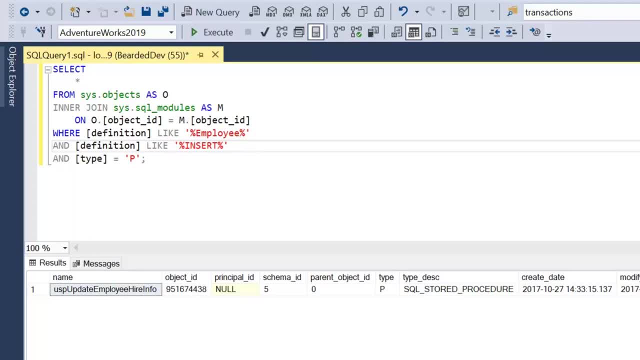 words. we'd have to be quite clever about what text we're actually writing and searching for, especially if we've got hundreds of stored procedures or other objects in this database. we don't have hundreds of objects, so it's quite easy to narrow it down, but that is a good way to search. the definition of a stored.